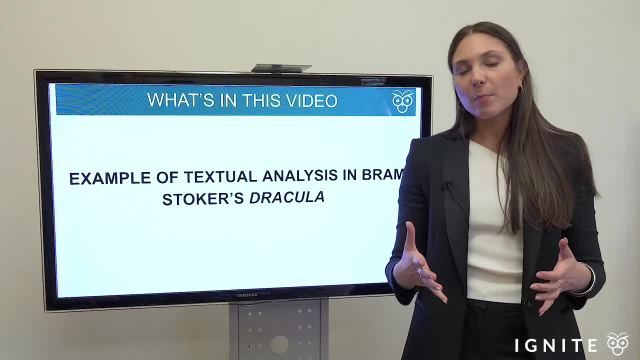 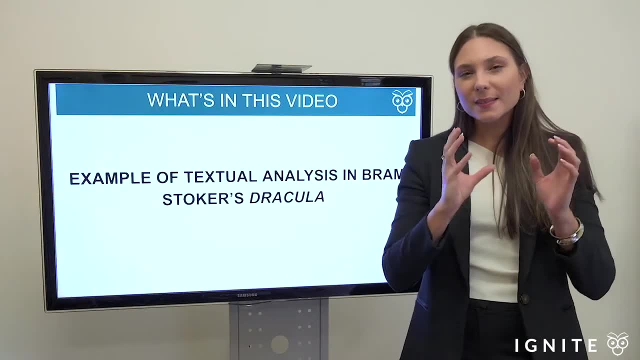 candid on the spot analysis on that for you guys. But my point in doing that is to reiterate in anyone doing any textual analysis's mind the steps that really must be undertaken in order to unpack how meaning has been conveyed. So let's get started. 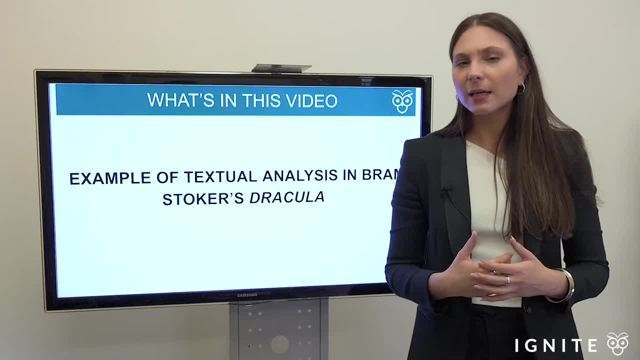 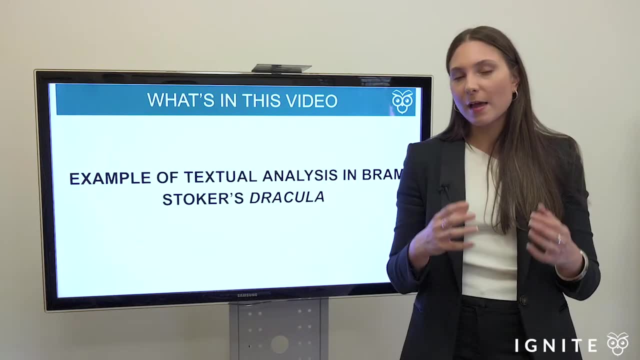 So if you're a younger student in particular and you're a little bit stuck with English and you're wondering, well, what's really the point in my English studies and what am I seeking to convey in my writing, this video will be particularly useful for you. I'm going to talk a little bit. 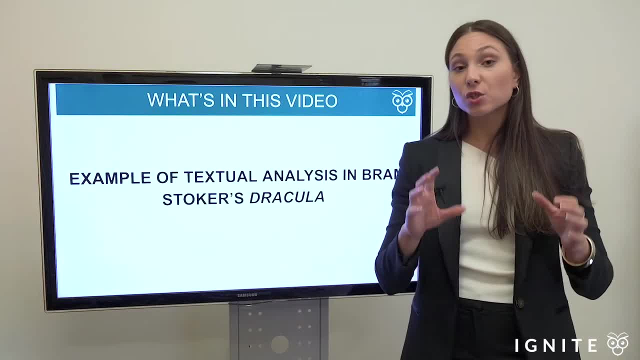 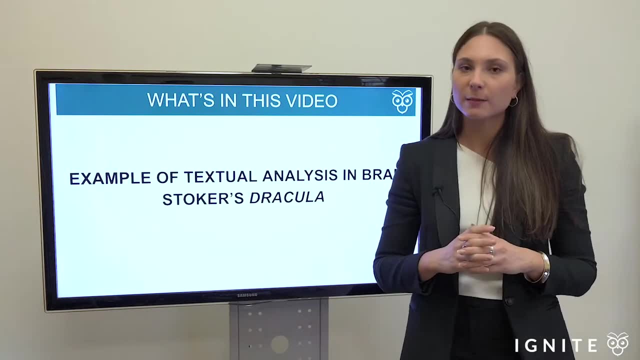 about what textual representation actually means, and then show you how to actively read an extract from a text in order to unpack how a composer is using those aspects of form and feature in order to convey some sort of impact on your writing. So let's get started. 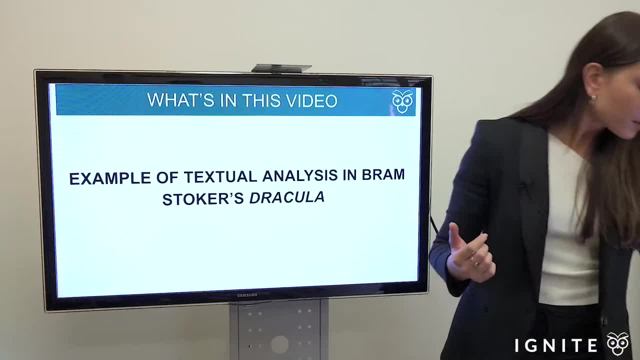 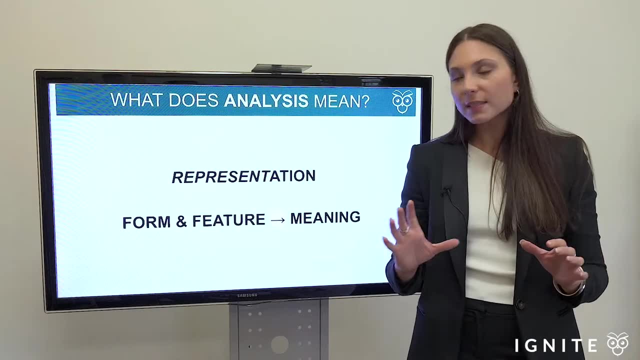 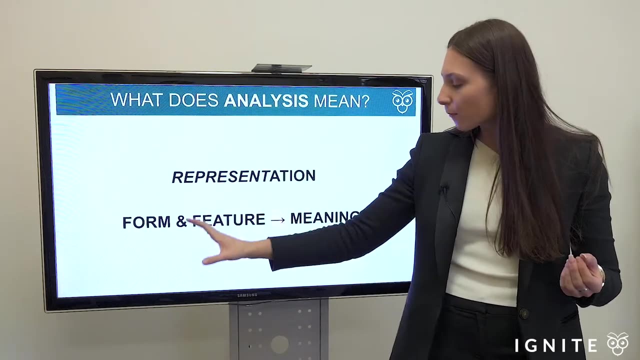 So when we're thinking about texts and we're looking at how ideas are conveyed in text, we're really asking ourselves: how is representation functioning in that text? Now, what that means is: how is the composer used, form and feature to convey meaning? Now, I've highlighted this arrow. 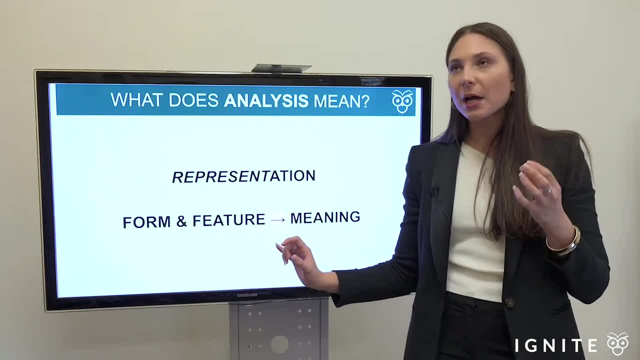 here because I'm trying to illustrate that, as a student, you can't just simply assert that meaning has been conveyed in the text. It's not just that you can't just simply assert that meaning has been conveyed in the text, It's that you can't just simply assert that meaning has been conveyed in the text. 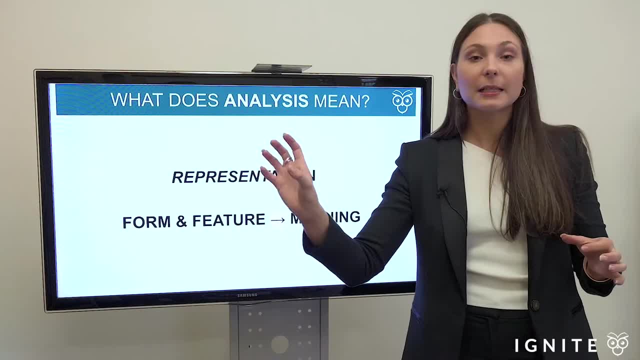 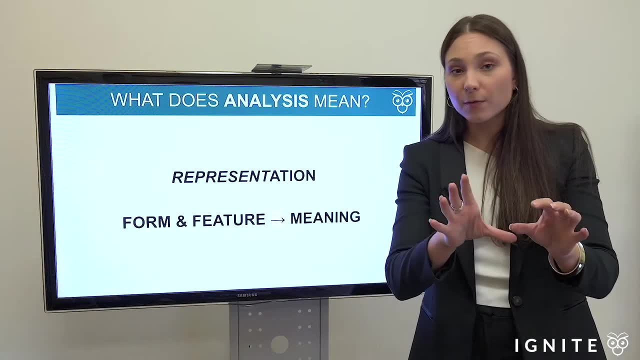 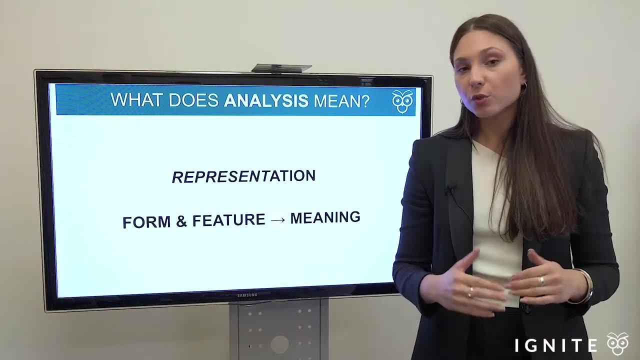 If you're saying here that a composer has explored this particular theme, or this quote evokes this idea, you're not actually justifying the assertion that you're making. You must get into the habit, and indeed it should be second nature for you to assert how the composer has. 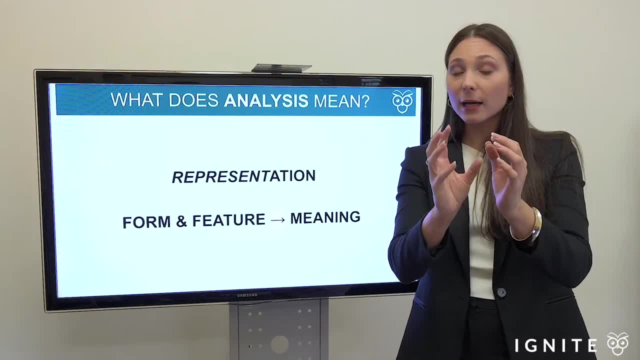 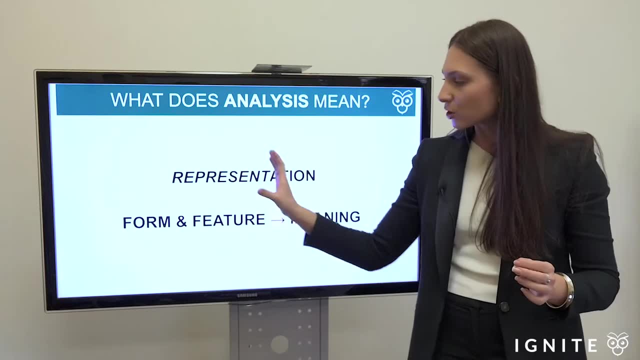 used a technique or an aspect of form in order to trigger their responder to appreciate that idea that is being conveyed. Okay, so that's what I'm going to show you here in my reading of the following extract. As we're going through, I'm going to actively pick. 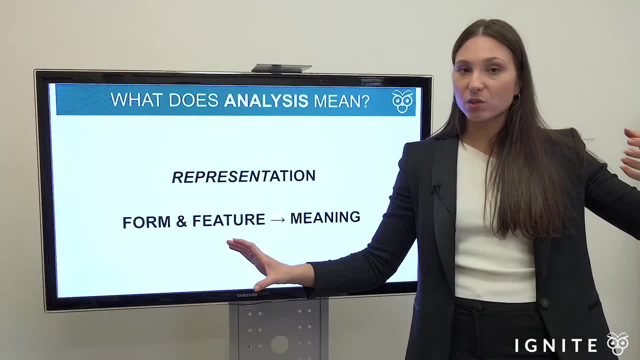 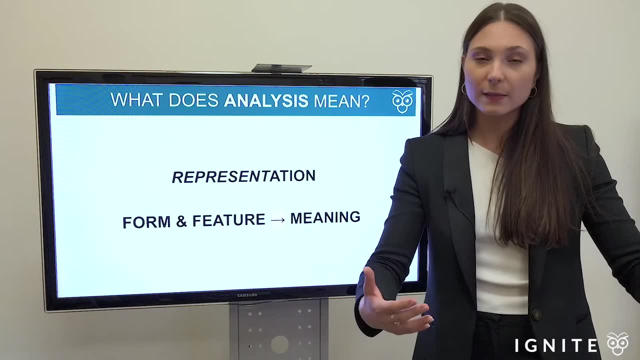 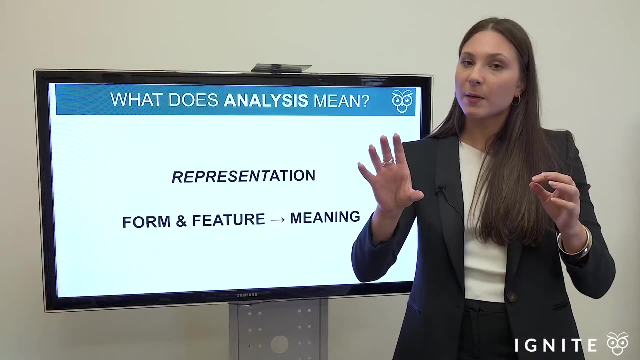 out the techniques that the composer has used in that extract and how that impacts me as a reader. to illustrate to you how, when you are writing your own forms of analysis, you get into the habit of taking out extract from the text or quote from the text identifying the technique or aspect of form. 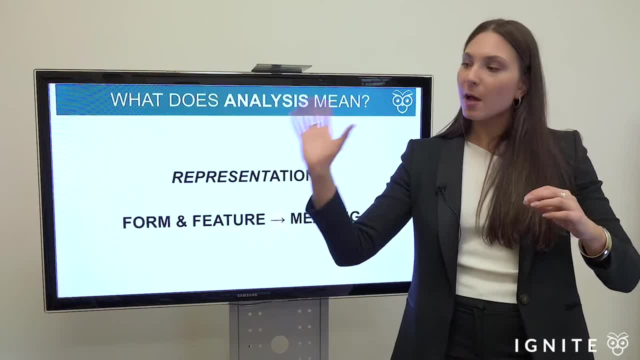 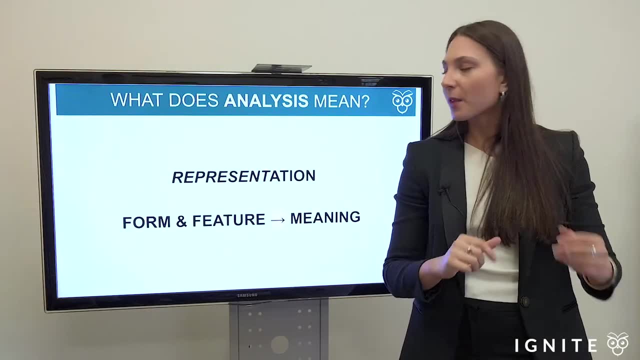 and then going on to say what the effect of that is Okay, but before we get to that effect, you must go back and ask yourself how that technique or aspect of form has impacted you. Okay, so I want to ask yourself: what technique or aspect of form has the composer used? Let's have a look at our. 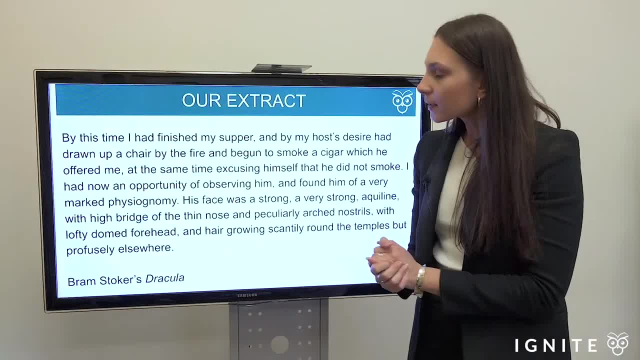 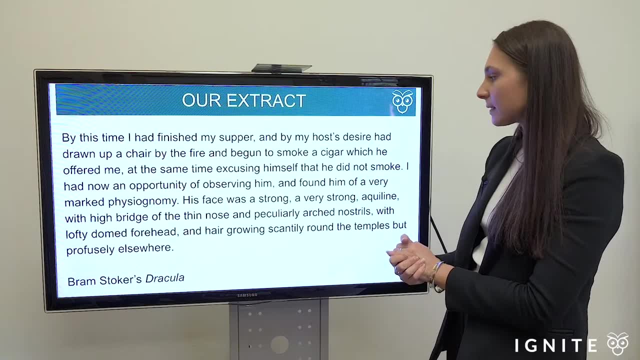 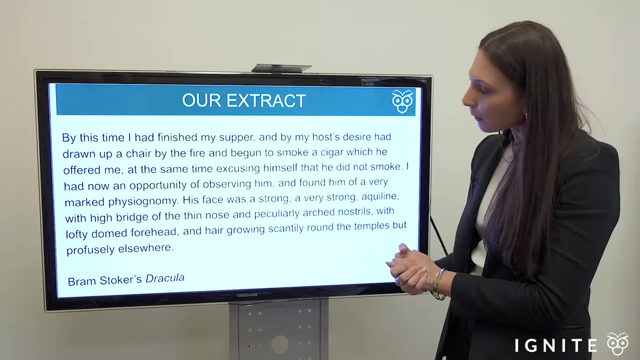 extract. By this time I had finished my supper and, by my host's desire, had drawn upon a chair by the fire and begun to smoke a cigar which he had offered me, at the same time excusing himself that he did not smoke. I had now an opportunity of observing him and found him of a very marked 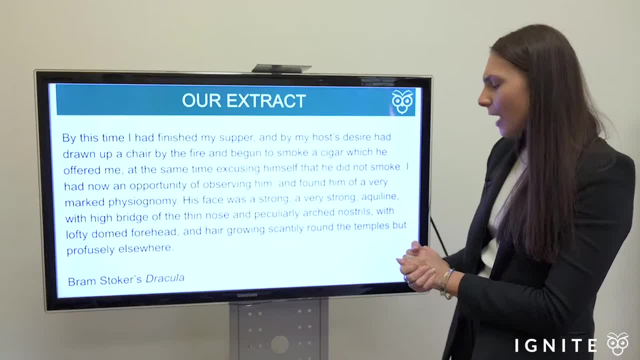 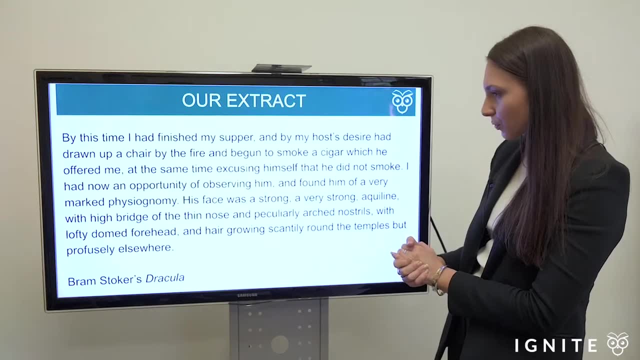 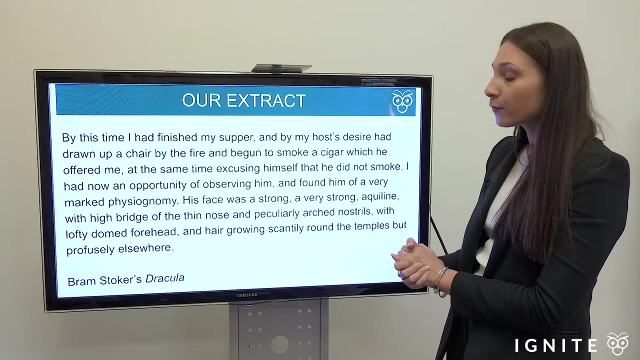 physiognomy. His face was a strong, a very strong aquiline with high bridge of the thin nose and peculiarly arched nostrils, with lofty domed forehead and hair growing scantily around the temples but profusely elsewhere. Okay, so that's the first read. Now just to kind of orientate you. 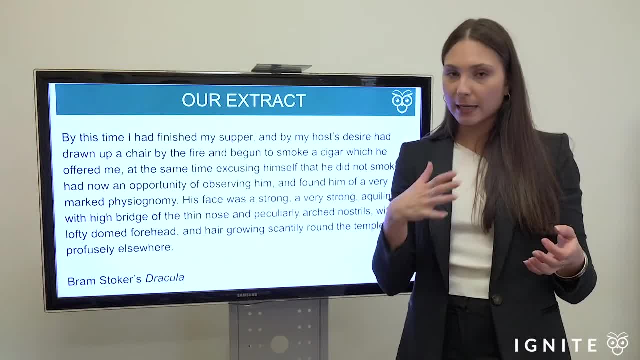 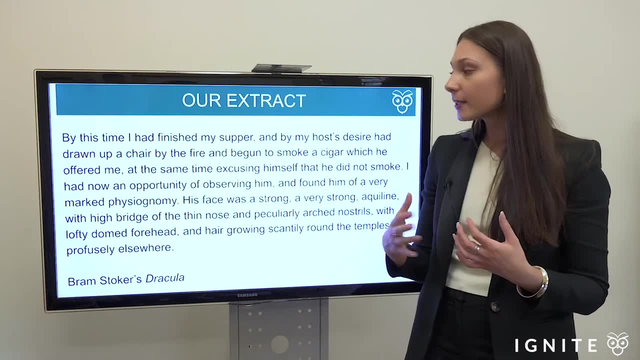 in the text. I've picked Stoker's Dracula because it's quite a popular text for students in years eight, nine and ten, particularly if you're a student of Stoker's Dracula. I've picked Stoker's doing a module on gothic literature or the late Victorian period and it's just a really great text. 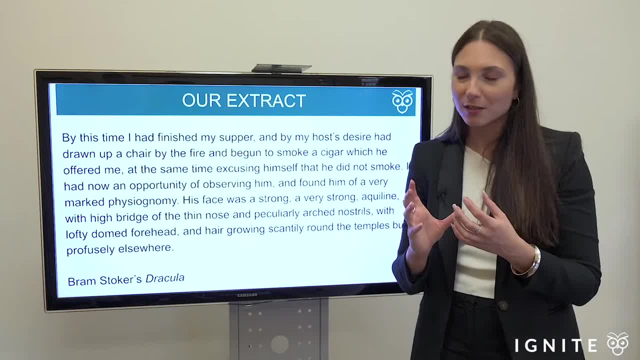 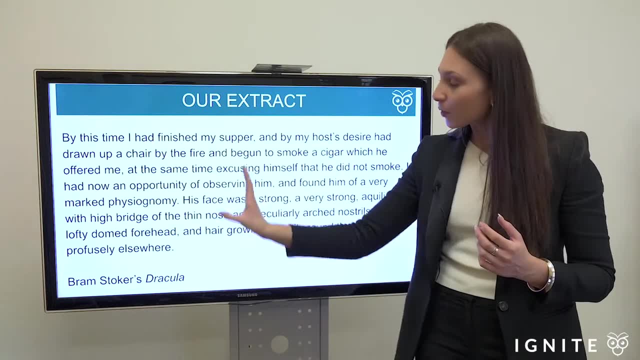 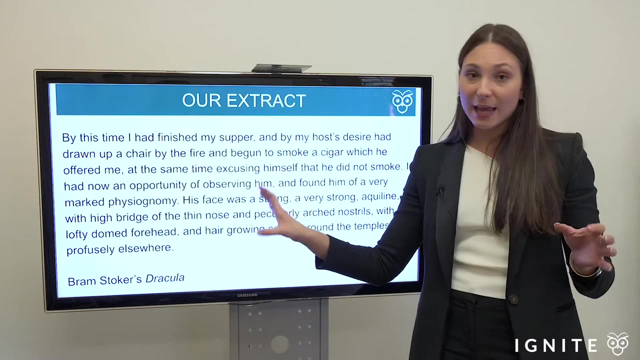 to read in terms of how the composer has used forms and features to convey this real, exotic otherness of Dracula. Now going back to orientating you in the novel, at this point our protagonist, who is Jonathan Harker, has arrived at the Count's property and he's starting to note some very 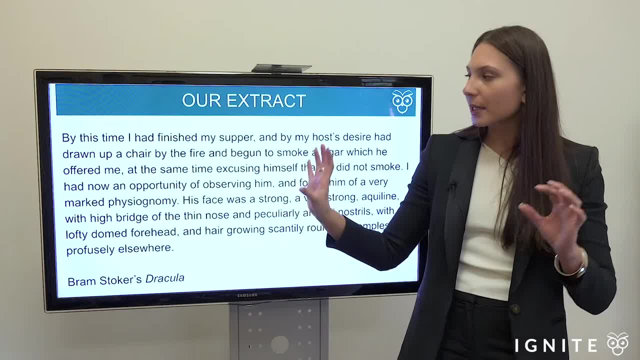 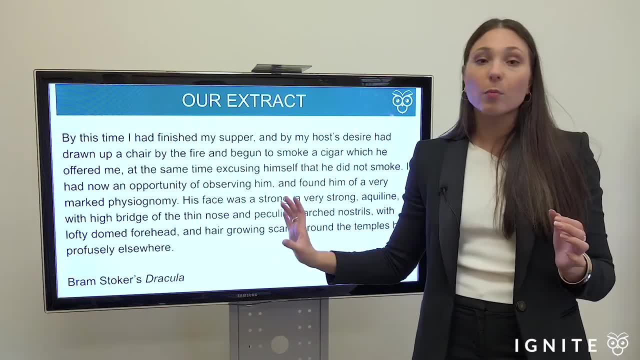 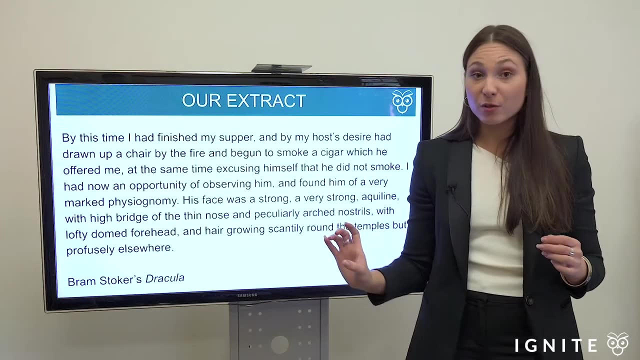 strange Easter European, if you will, exotic otherness about this location, but particularly in the characterisation of the Count as almost animalistic or what we would call zoomorphic. So let's have another read through and start to unpack what techniques have been used in the extract. So we have 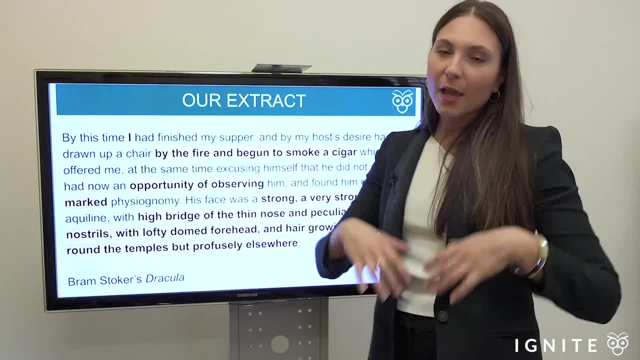 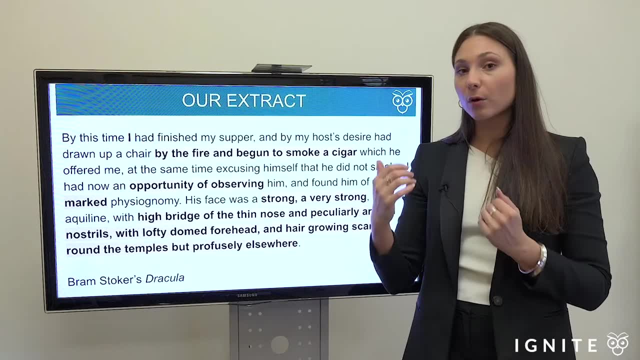 by this time I had finished my supper. Whenever you're doing analysis and you're seeking to assert that you, as a reader, has engaged a person who is not a reader, you're not a reader. you're not a personal dialogue with the narrator. you can comment on first person narration, The. I invites. 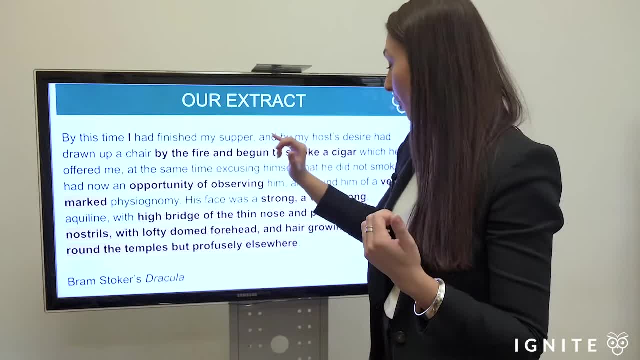 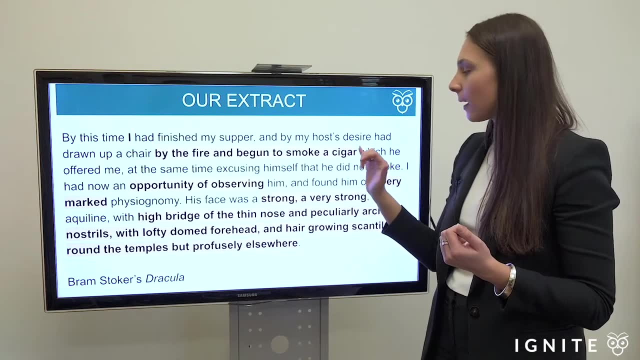 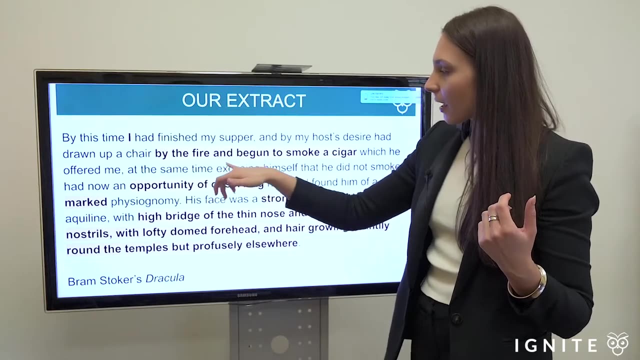 us into intimate dialogue with the composer And by my host desire had drawn upon a chair by the fire and begun to smoke a cigar. This here is very effective in conveying setting to the reader. The fire conveys a sense of imagery and begun to smoke a cigar also appeals to 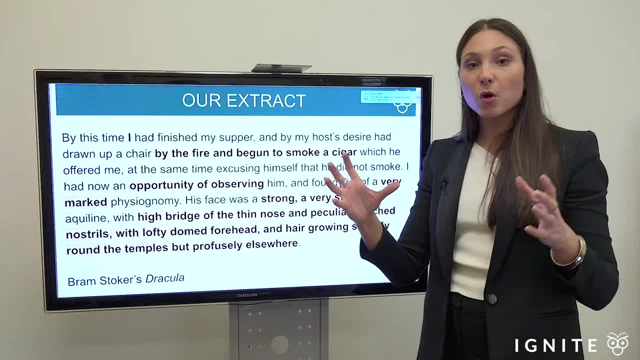 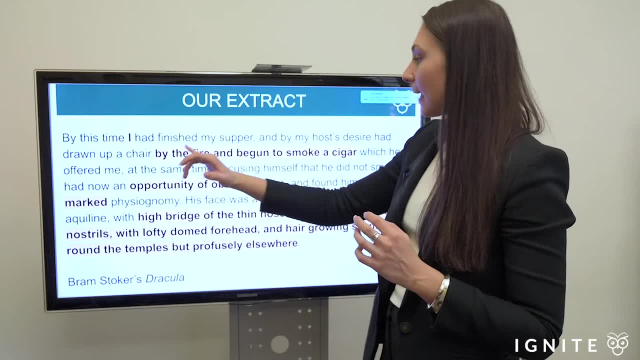 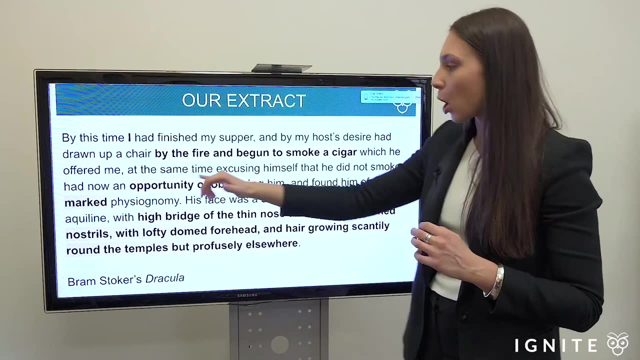 olfactory imagery, which is smell, to give us a strong sense of both the temperature and the smells that constitute the surroundings, which he offered me, at the same time excusing himself that he did not smoke. I had now an opportunity of observing Opportunity and observing the 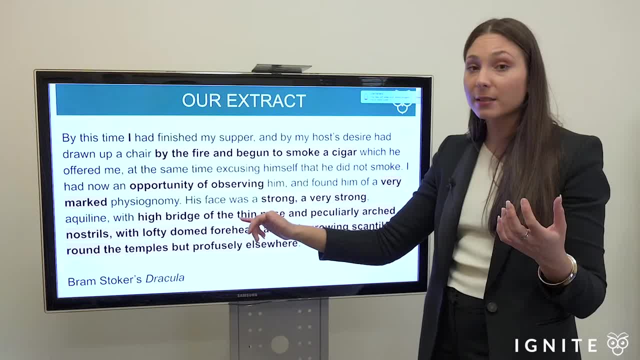 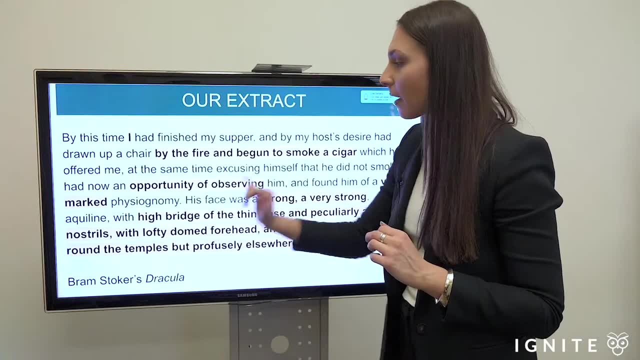 repetition of the O is a form of alliteration, drawing our attention to how astutely Jonathan Harker is watching the Count and found him of a very marked physiognomy. Very marked, see the assertion in what's being conveyed there and the level of certainty. 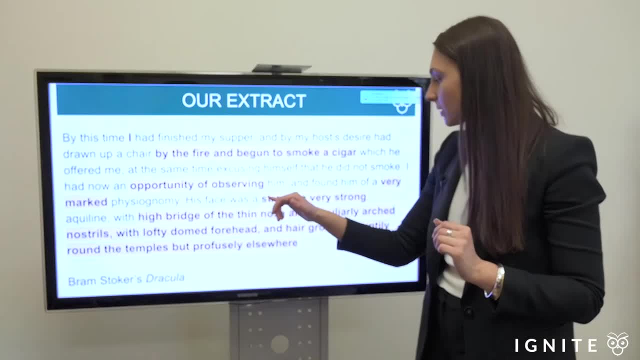 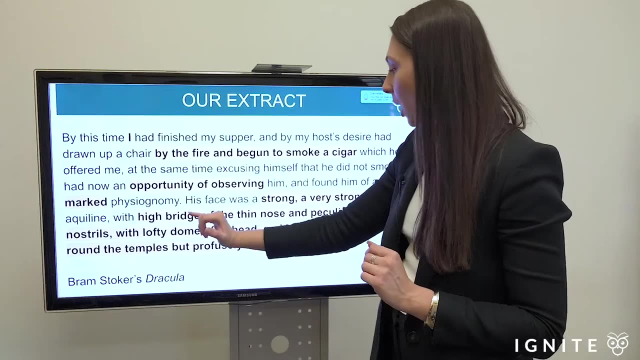 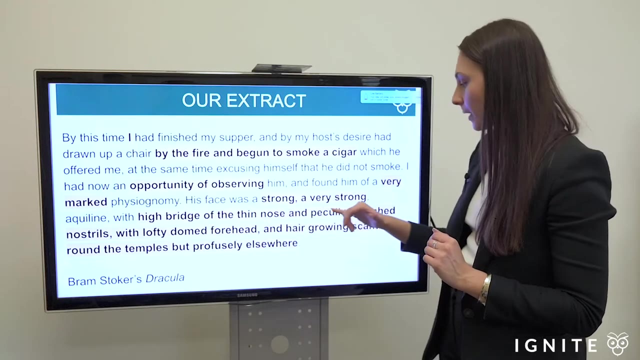 we call that high modality. His face was a strong, a very strong repetition there, reinforcing the strong nature of his face, aquiline with high bridge of the thin nose and peculiarly arched nostrils. So again here, visual imagery is being used to convey the 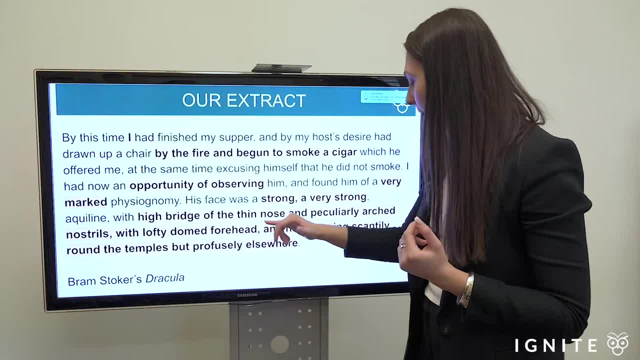 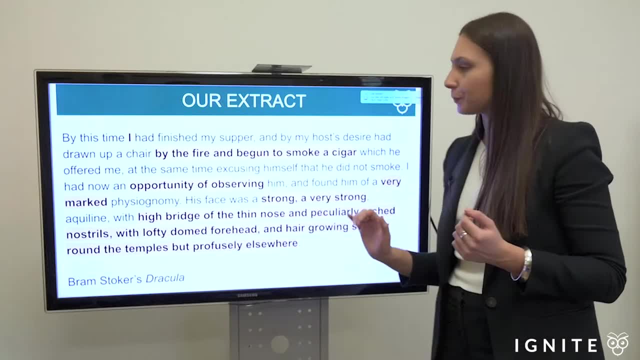 appearance of the Count with lofty domed forehead and hair growing scantily around the temples but profusely everywhere else, And the imagery is continuing there too. So what I'm hoping you guys have taken away, as I've read through that extract, is how you actively 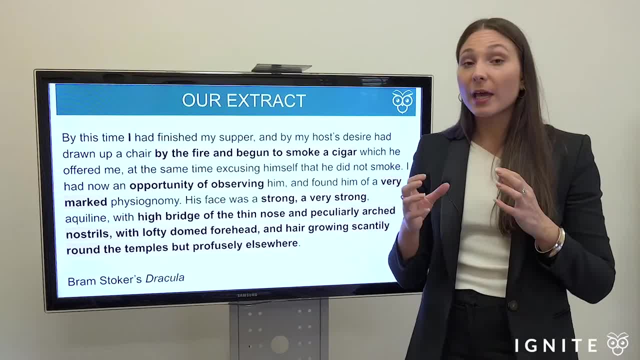 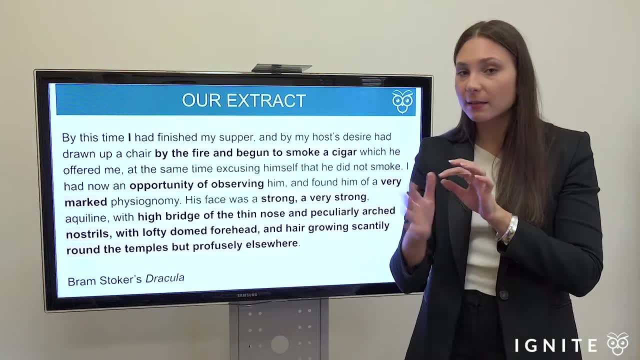 read through portions of the text and you ask yourself, okay, what techniques are being used? Setting, characterization, visual imagery, narrative voice and modality are always good places to start. So if you are watching this as a younger student and you want to kind of build on, 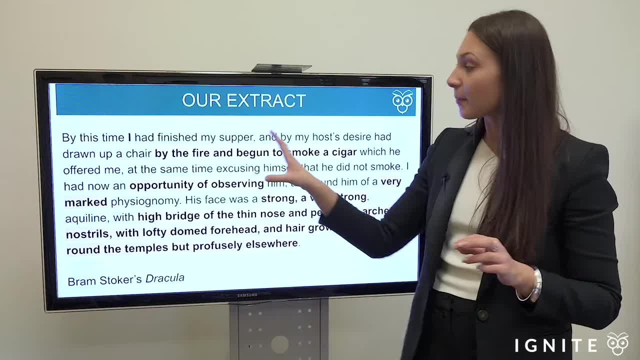 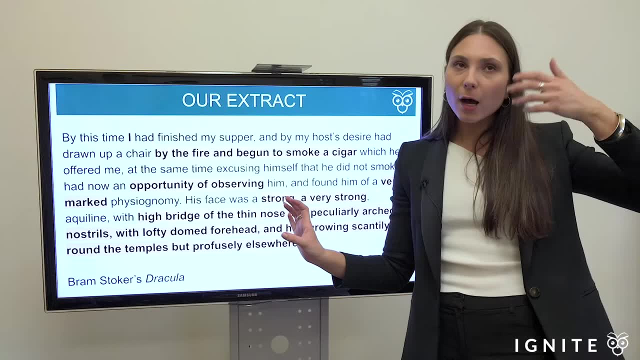 your bank of techniques. take note of all the things that are being used to convey the image, All of the techniques I mentioned as I was reading through this, and just also note how, as we're reading through, we're actively asking ourselves: how is Stoker, or any composer, using those aspects? 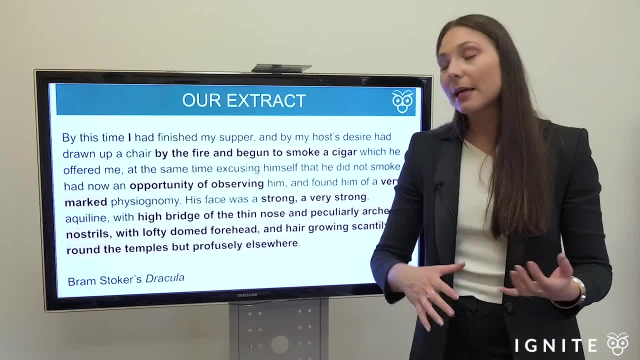 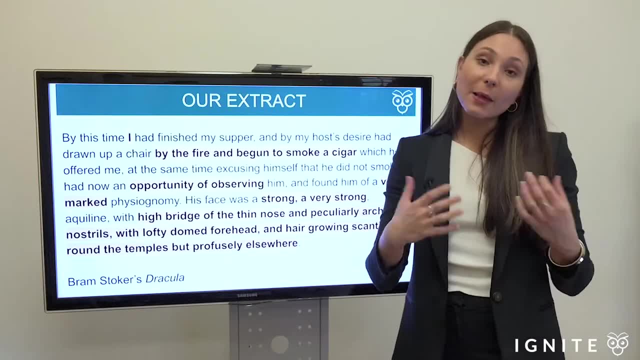 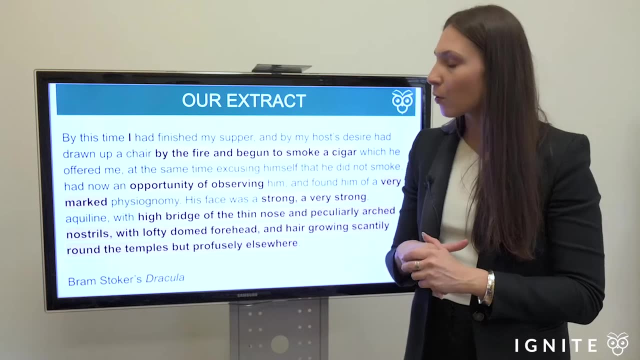 of form and feature to impact us in some sort of way. In this extract we've gotten a strong sense of the setting and a strong sense of the characterization of Dracula, and that's been done through the techniques that Stoker has used. Okay, guys, that concludes my analysis for